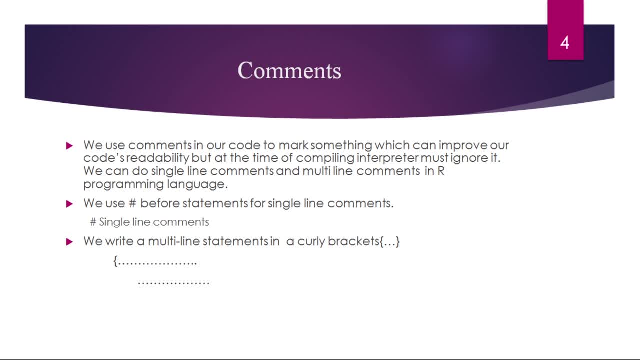 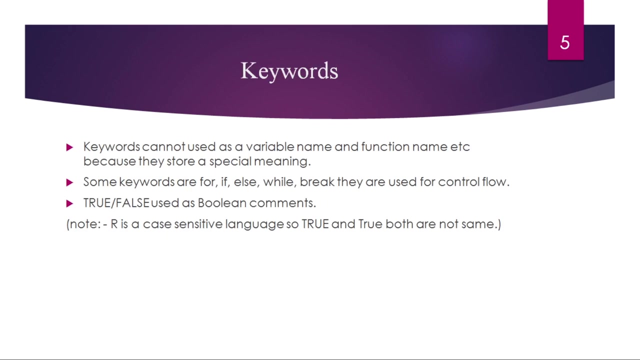 line commands. in R We use hash hashtag before statements for single line commands And use a curly bracket and a double quote for a multi-line statements for a multi-line comments. now keywords. keywords can cannot used as a variable name and function name because the storage specific meaning some keywords are for. 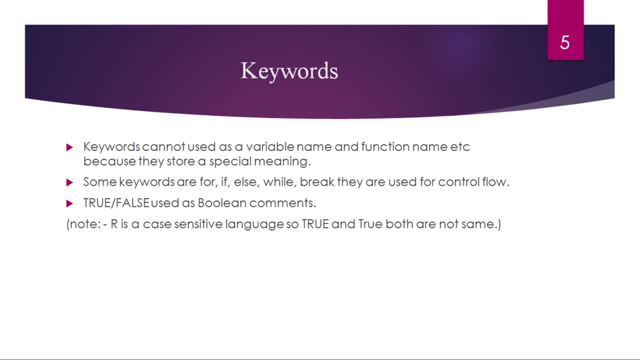 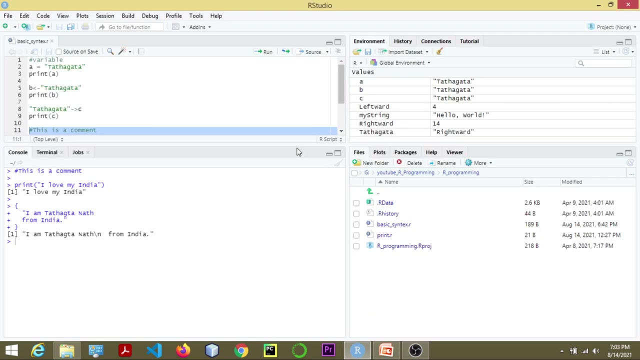 some keywords are for if else, while break they are used for control flow. capital true or capital false, used as boolean comments. note that are is a case-sensitive language, so capital true and true, both are not same. now I take my name to some practical first variables. take a very well a and store a string. I take my name. 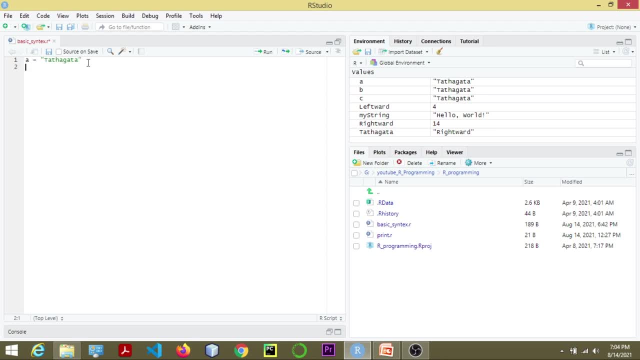 field name is printing and A will get you a Layout. it appear A print a. it show me the my name. this is the output, my name now first clear it, then run again. yes, hospital is my name. operator where data are copied from right to left in simple variable data's are copied. 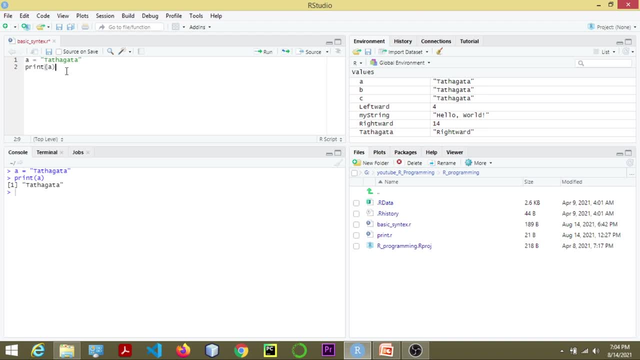 from right to left. Similarly, leftward operator- also copied data from right to left. ok, I take a variable b and put a string. I also take my name with a title, then print my full name, select this two line and run. Yes, it show me my full name. then rightward operator. rightward operator- copied data from. 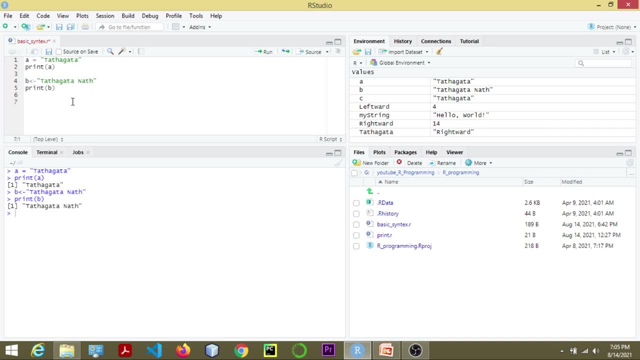 left to right. ok, so first I take a string: my nation name. my country name, India. ok, I take a string and store it. a variable c variable: print it first, select both two line and run. yes, sorry, I do a mistake, I put my country name wrong. sorry, yeah, India. 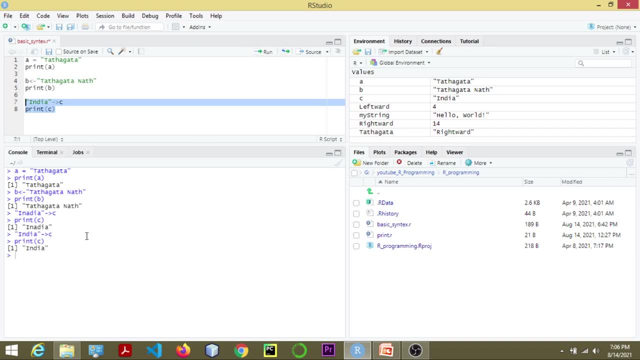 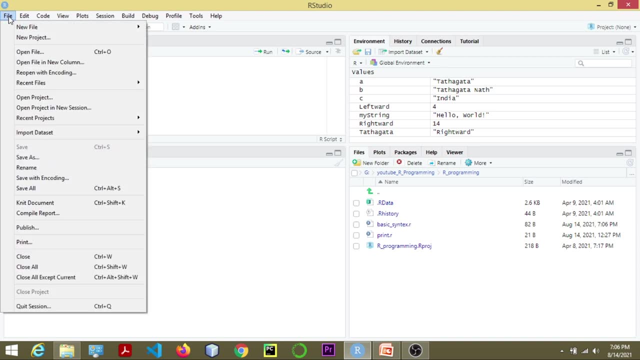 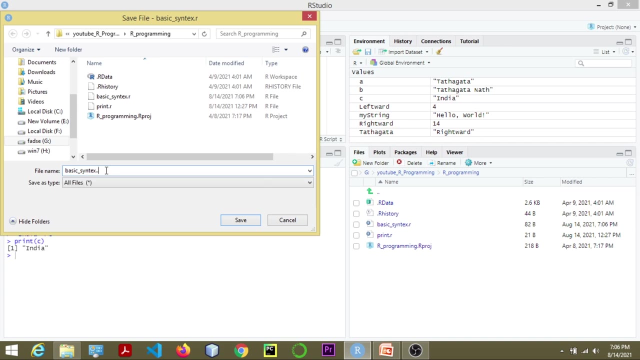 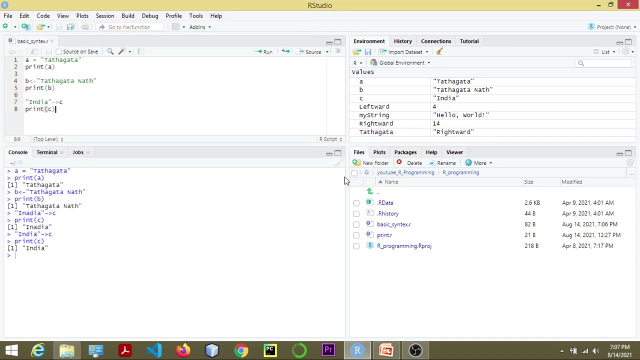 Ok, Ok, Now I save this file. save as basic syntax: dot r. r is the extension name. save. ok now comments. Ok, Ok, Ok, Ok, Ok, Ok. Ok For single line comments. I use a hashtag before the statement. I am Tathagata print variable.